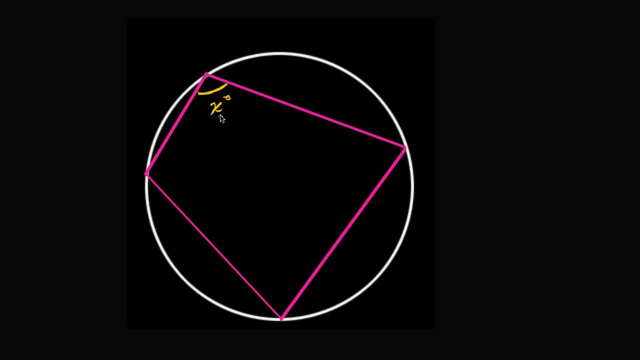 It's going to involve the measure of the arcs that the various angles intercept. So let's think about it a little bit. This angle that has a measure of x degrees, it intercepts this arc. So we see, one side of the angle goes and intercepts. 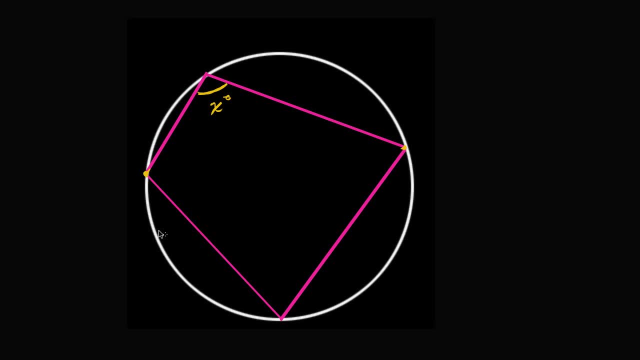 the circle there, the other side, right over there, And so the arc that it intercepts, I am highlighting in yellow, I am highlighting it in yellow, Trying to color it in. So there you go. Not a great job at coloring it in, but you get the point. 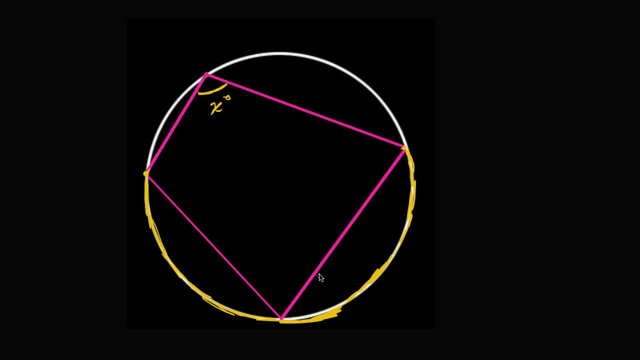 That's the arc that it intercepts, And we've already learned in previous videos that the relationship between an inscribed angle- the vertex of this angle sits on the circle- the relationship between an inscribed angle and the measure of the arc that it intercepts. 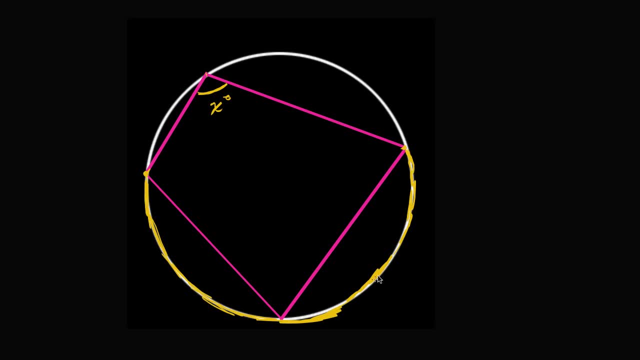 is that the measure of the inscribed angle is half the measure of the arc that it intercepts. So if this angle measures x degrees, then the measure of this arc is going to be 2x- 2x degrees. Alright, well, that's kind of interesting. 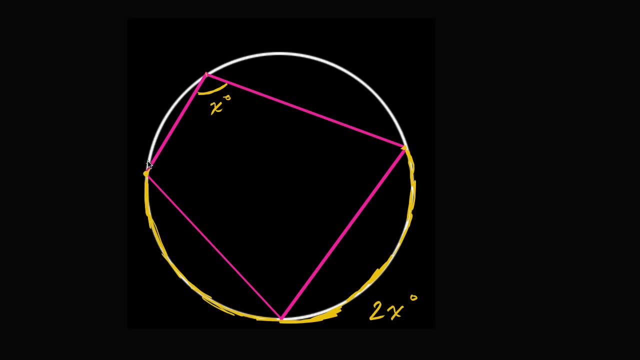 but let's keep going. If the measure of that arc is 2x degrees, what is the measure of this arc right over here, the arc that completes the circle? Well, if you go all the way around the circle, that's 360 degrees. 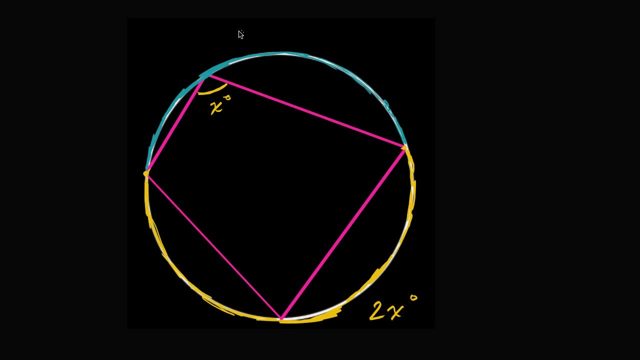 So this blue arc that I'm showing you right now, that's going to have a measure of 360 minus 2x, Minus 2x, Minus 2x degrees, 360 is all the way around. The blue one is all the way around, minus the yellow arc. 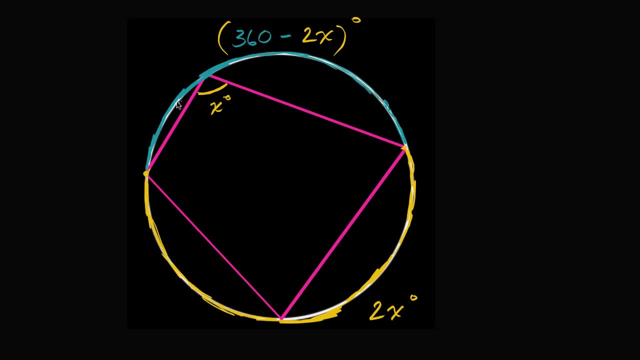 What you have left over, if you subtract out the yellow arc, is you have this blue arc. Now, what's the angle that intercepts this blue arc? What's the inscribed angle that intercepts this blue arc right over here? What's this angle? 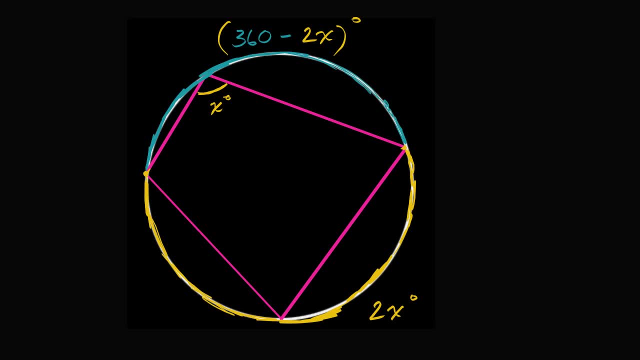 It's the angle that we wanted to figure out in terms of x, It is. it is well, I'm having trouble changing colors. It is that angle right over there. Notice the two sides of this angle. they intercept this angle, intercepts that arc.